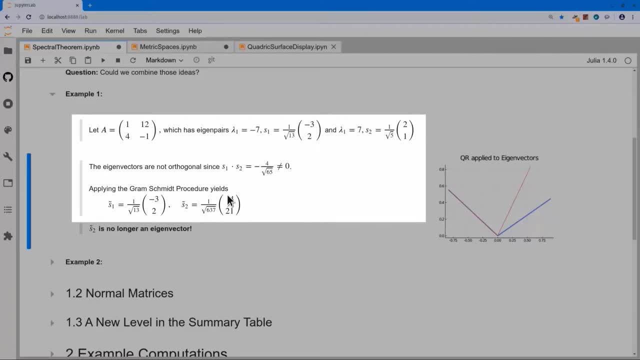 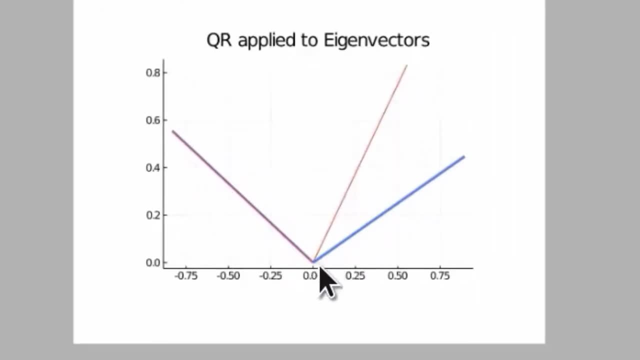 still lies along the original direction, but the second vector got replaced by a new vector. Here's the picture. I started with the red vectors. The red vectors are s1 and s2.. They are not orthogonal to each other And now I replaced s2,, this vector, by its orthogonal projection, instead of the. 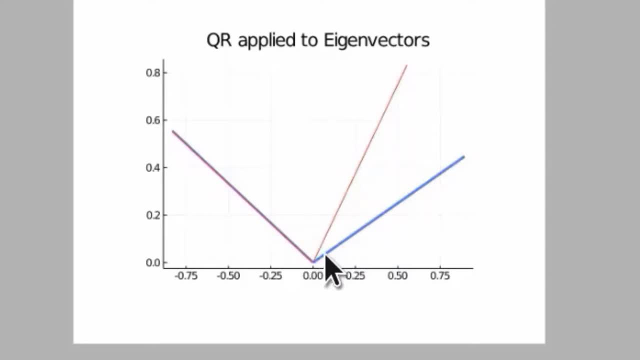 original vector to get a right vector. But now this new vector is no longer in the direction of either one of those eigenvectors. It's an entirely new direction, And so applying a to this particular vector is not going to have the property that ax is equal to line. 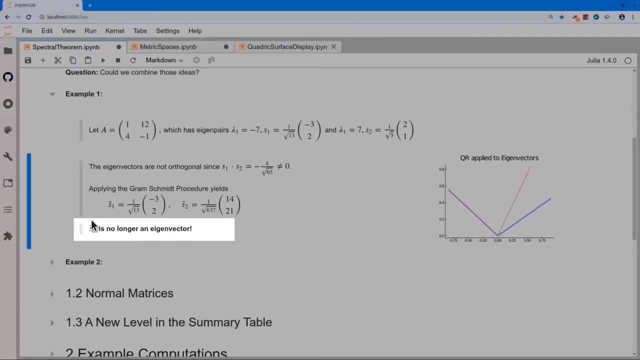 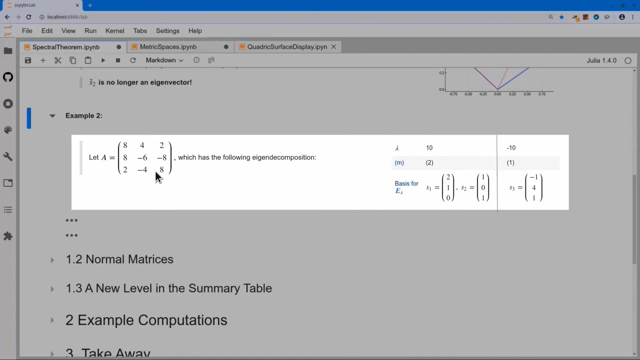 It's going to be lambda x for some lambda, So this new vector here is no longer an eigenvector. It sounds like bad news. It sounds like I can't apply Gram-Schmidt. However, that's not quite true. Look at this new matrix here: A and I've computed the eigendecomposition. 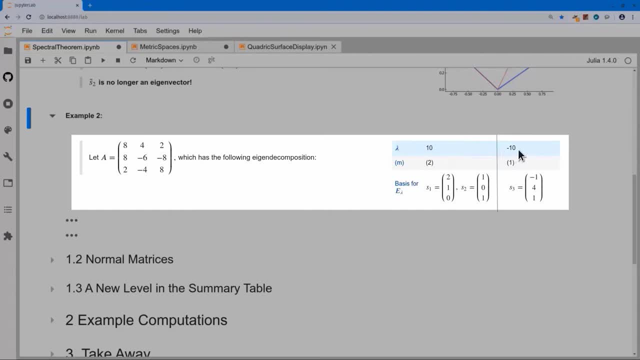 This is what I see. It's got two eigenvalues: an eigenvalue of 10 and an eigenvalue of minus 10.. For the eigenvalue 10, 10 occurred twice, And so I've got two vectors in the basis. 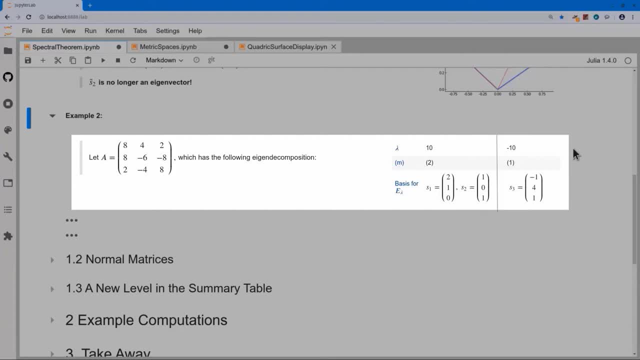 I've got a plane corresponding to eigenvalue 10.. So for the other eigenvalue minus 10, I have dimension 1 for the corresponding eigenspace. So I need a single basis vector. And if you look at this basis vector it happens to be orthogonal to s2.. That dot product between. 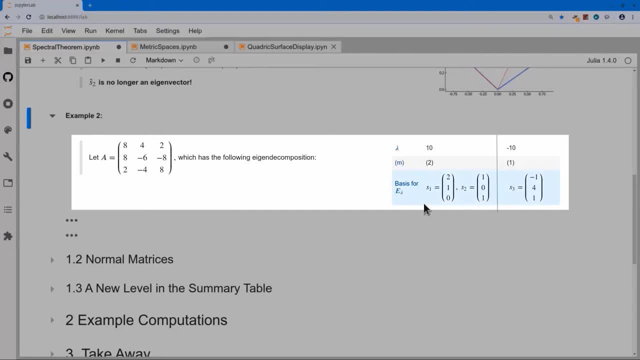 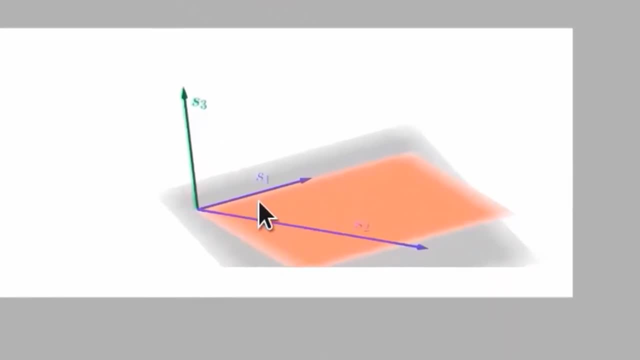 s2 and s3 is 0. But it's not orthogonal with s1.. However, if I think about Gram-Schmidt. so here is an example. I've got my s1 and s2.. They form a plane. The eigenvalue for this plane is 10.. And then I have an s3 vector And it sticks out from. 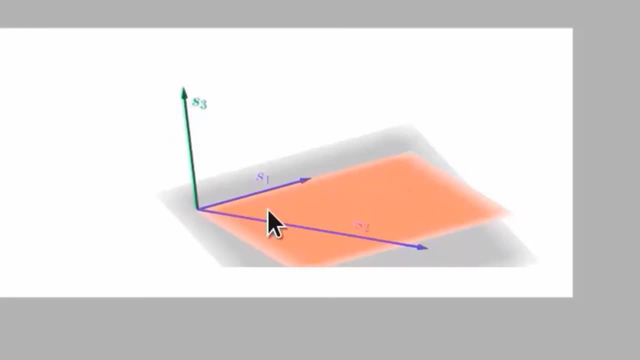 that plane S3 happens to be orthogonal to s1, but it's not orthogonal to s2.. But within the plane s1 and s2, if I do Gram-Schmidt, all I'll do is I'll take this s2 vector and 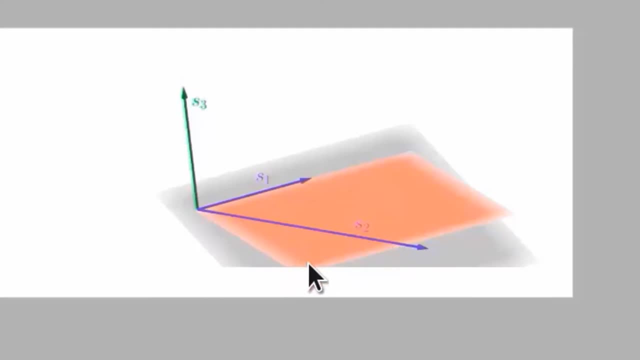 I'll straighten it out. I'll get it along this edge of the plane over here And it's still going to be an eigenvector And s1 and s2 still will define the eigenspace and a linear combination of the eigenvectors. 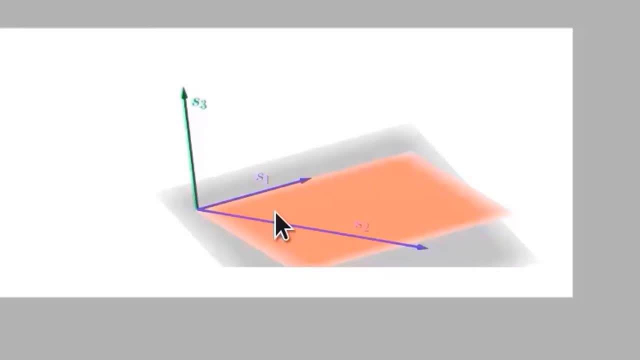 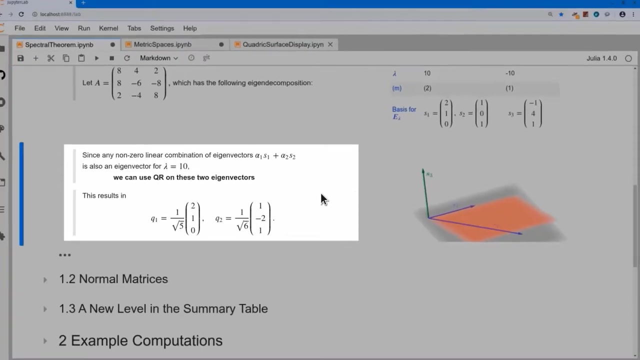 Those new vectors will still be an eigenvector for lambda equals 10.. I just can't combine Gram-Schmidt. I can't do Gram-Schmidt for different eigenvalues because that would get me away from the eigendirection. So any non-zero linear combination of the original eigenvectors s1. 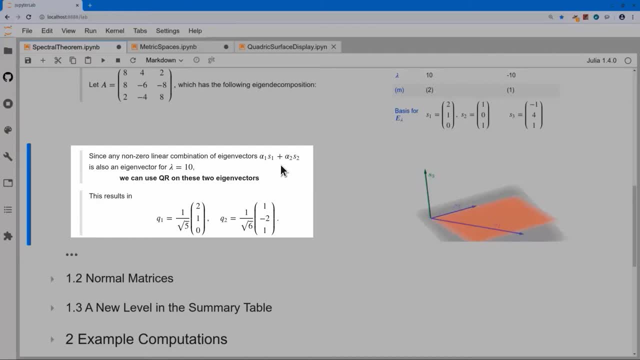 and s2 for lambda equals 10 gives me another eigenvector, And so, using QR these two vectors, a unit vector along the s1 direction plus an orthogonal unit vector in that red plane, gives me a basis for the eigenspace with lambda equals 10.. That works. I just can't go across. 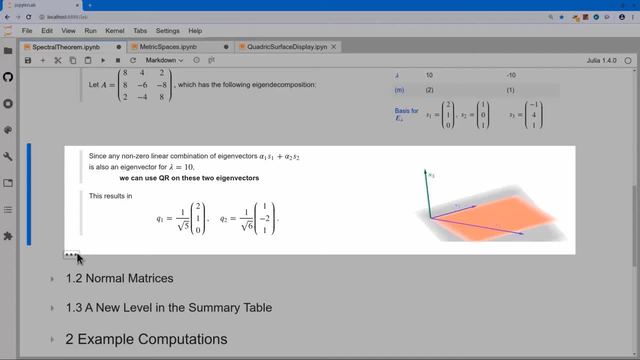 different eigenvalues. Now if I ran the problem in reverse, I could start with orthogonal eigenvectors and get some lambda matrix and multiply it all out. I would have an orthogonal set of eigenvectors. So I know it exists. The question that arises then is: under what conditions are we lucky? 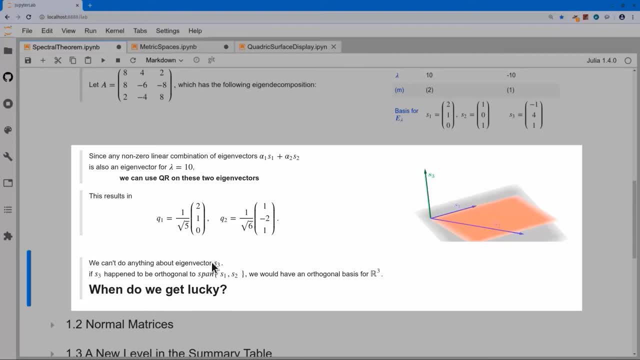 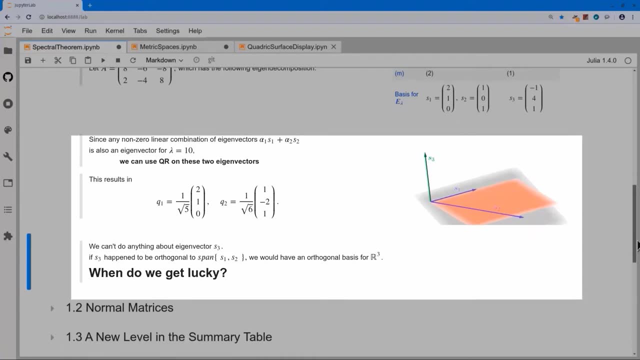 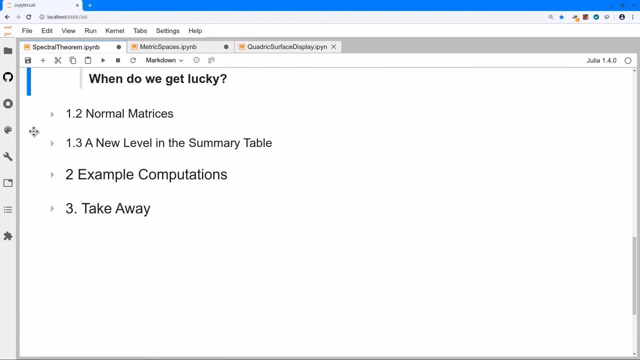 Under what conditions would this eigenvector s3 happen to be orthogonal to the eigenvectors s1 and s2?? Because then I would indeed end up with an orthonormal set of eigenvectors with a basis for all of R3.. So when do we get lucky? The answer to that question comes. 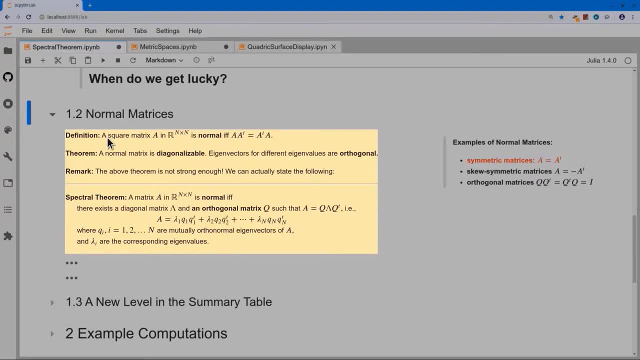 from what are known as normal matrices. Okay, And specifically, there are matrices such that A times A transpose happens to be the same as A transpose A. So if those two products are the same, we call that a normal matrix and it gets a special name, Because if that's true, then that matrix is diagonalizable. 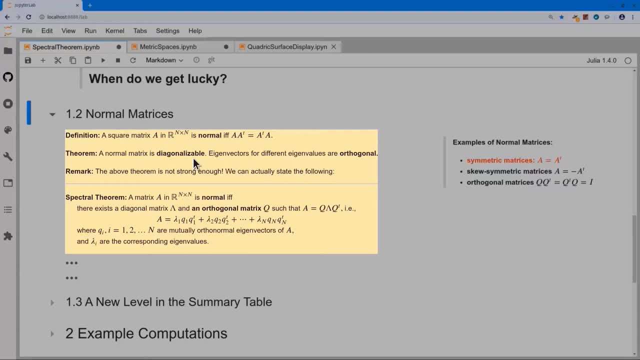 And not just that, but the eigenvectors for the different eigenvalues are also there. I wrote it out as a separate theorem because that's the fact that we really are going to be using it. But that theorem is actually not strong enough. I can make a much stronger. 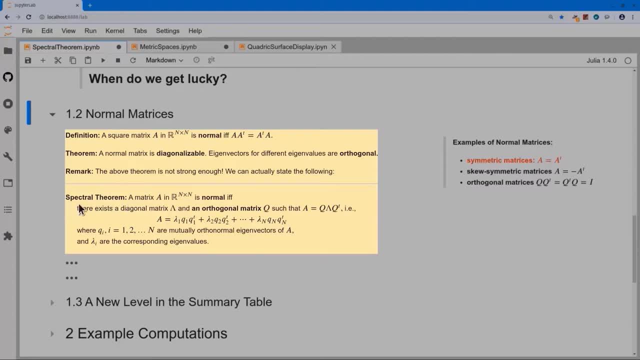 statement. It's called the spectral theorem. The word spectrum is associated in mathematics with the eigenvalues of a matrix. So a matrix A has a spectrum. It has a certain set of eigenvalues. If I start with a normal matrix A, then the theorem says: I can diagonalize A, So there, 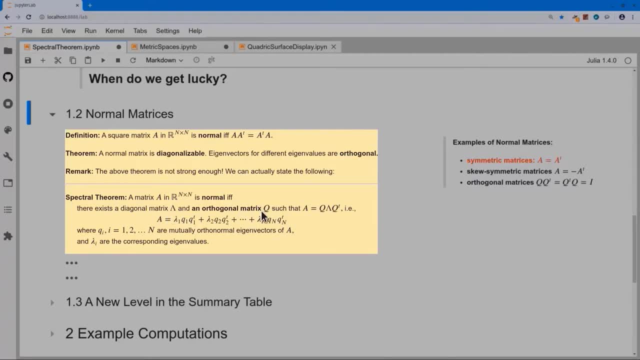 is a diagonal matrix, lambda it, I can diagonalize it with orthogonal eigenvectors, And therefore my eigenvector matrix, which used to be coalesced traditionally, we now call it Q, when the eigenvectors are mutually orthonormal, So that matrix Q, therefore its inverse, is the transpose of Q, And so our 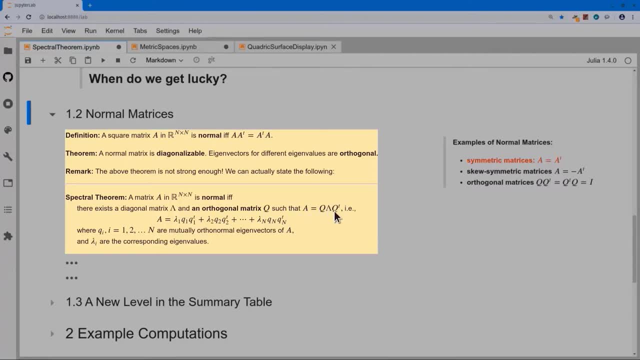 eigen decomposition now looks like A is equal to Q lambda, Q transpose. And if I try and multiply this out, I see that A looks like for each one of the eigenvectors: Q1,, Q2,, Q3, it looks like A. 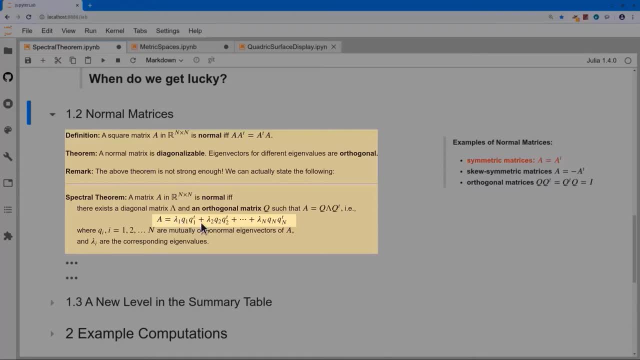 is equal to lambda 1, Q1, Q1 transpose. lambda 2, Q2, Q2 transpose. lambda n, Qn, Qn, transpose. And if you think back about the projection matrices in the special case when we had 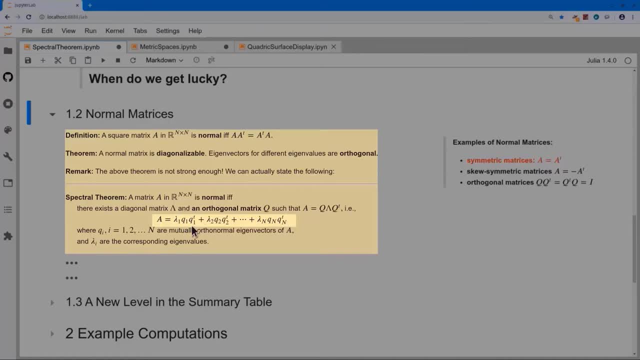 mutually orthonormal eigenvectors. you'll recognize these terms: Q1, Q1 transpose as projection matrices onto Q1, Q2, Q1 transpose The direction. Q1, Q2, Q3 transpose the orthogonal projection matrix onto Q2,. 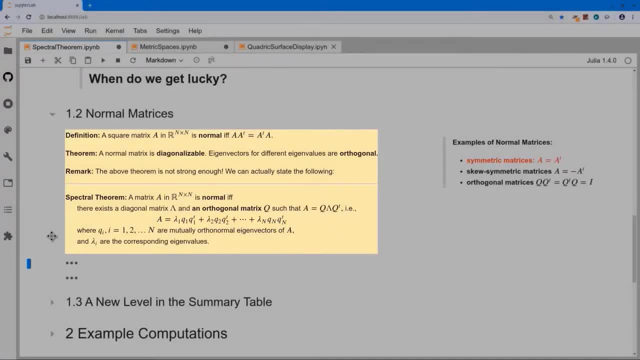 each one of these is an orthogonal projection matrix And the lambdas are the corresponding eigenvectors. Now, what kind of matrices are normal? So here are examples of normal matrices. The first, the important class of normal matrices, is symmetric matrices. 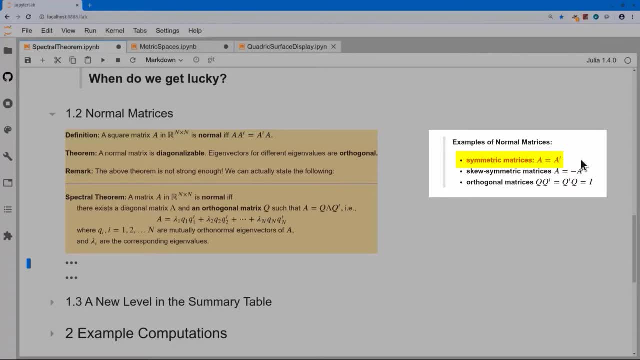 If A is equal to A transpose, if my matrix is symmetric, then A A transpose is A squared and A transpose A is A squared. Yeah, that matrix is normal Skew symmetric matrices. when A is equal to minus A transpose, they're also normal Orthogonal. 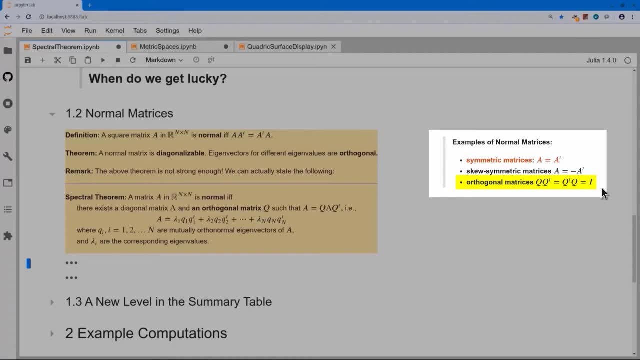 matrices. well, Q, Q transpose is I, Q transpose Q is I, so they're also normal. There are also examples of matrices that don't fall in any one of these classes, that are not symmetric, not skew, symmetric, not orthogonal matrices. It just can happen that some given matrix happens to be. 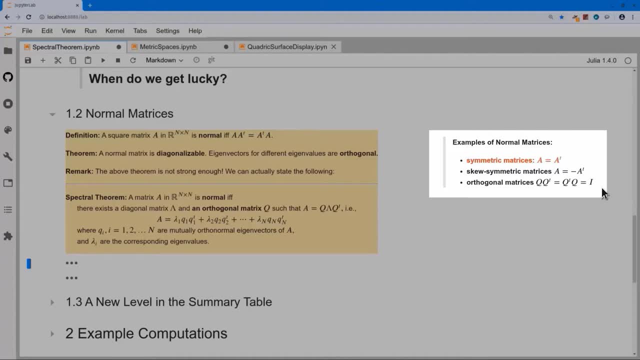 normal And therefore A transpose A is A squared and A transpose A is A squared. That matrix is normal. Therefore, A transpose A is a complete set of orthogonal eigenvectors. The couple of remarks that I want to make: the first one I already did. 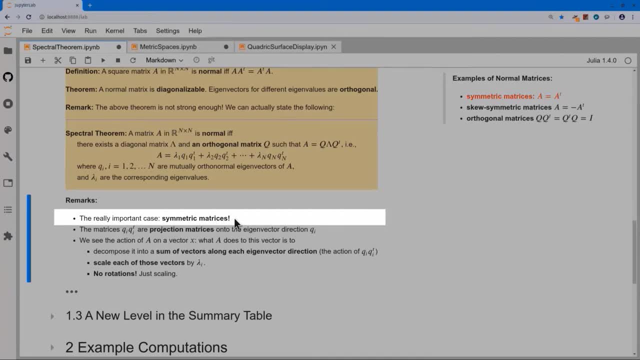 but I want to emphasize it again- is that the most important case is symmetric matrices. So if I have a symmetric matrix and if I look at the spectral theorem, at that expansion, what I see is projection matrices onto the eigenvectors Q. 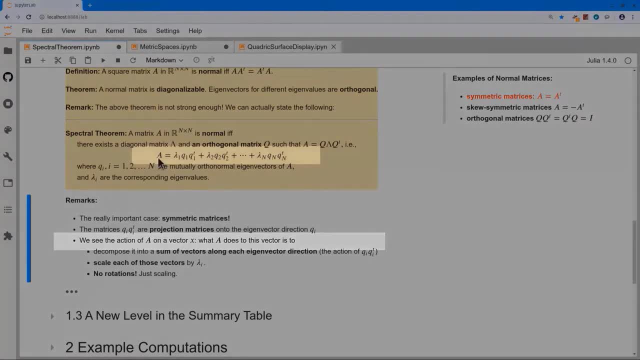 And therefore we also see the action that A has on the vector Compute. A times some vector. I'm going to get the orthogonal projection of that vector onto Q1, the component along Q1, and it's going to get scaled by lambda one. The orthogonal projection onto Q2 gets scaled by lambda. 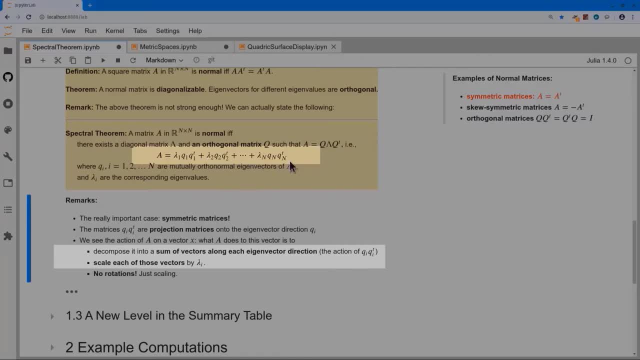 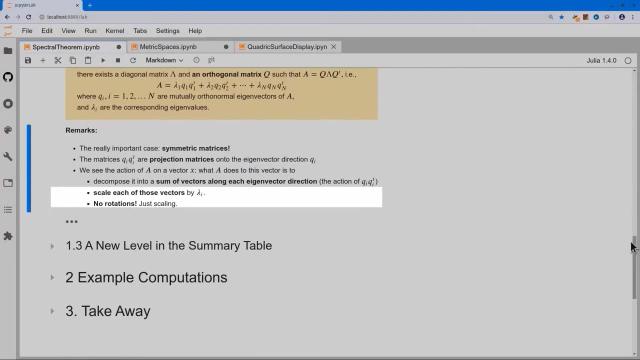 two et cetera. So we see what we already know, that matrices A that are diagonalizable do. they scale the eigenvector components by the corresponding eigenvalue. The other thing about this definition here is that this happens over Rm. We don't have any complex numbers that come in here. 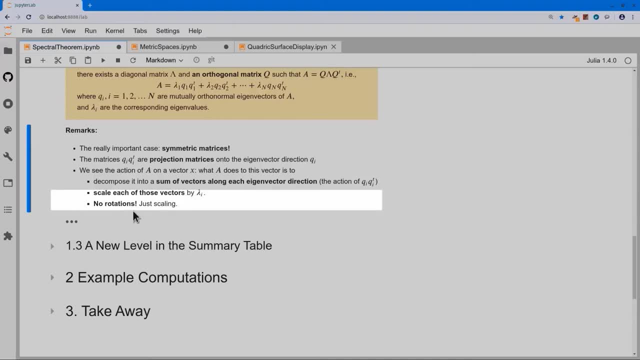 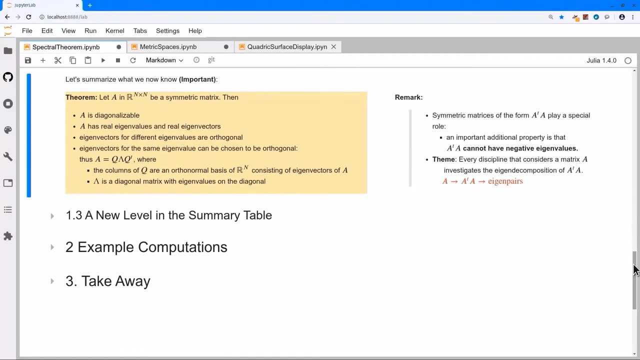 It's just scaling, no rotations that we had in the general case. So symmetric matrices. now let's summarize what we know about symmetric matrices. We've just added to it. If I start with a symmetric matrix, we already knew that A is diagonalizable. 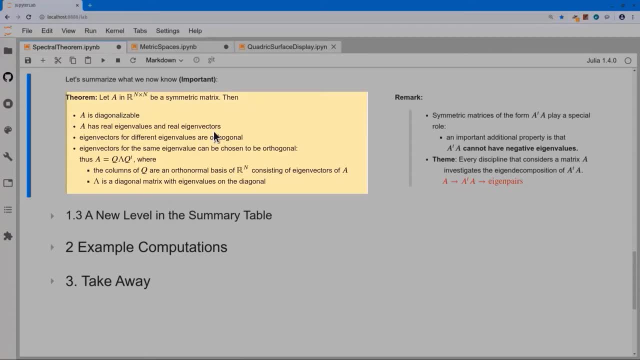 We already knew that it had real eigenvalues and real eigenvectors. Now we know that eigenvectors for different eigenvalues are orthogonal And eigenvectors for the same eigenvalue. if those null-space vectors we're computing don't happen to be orthogonal, we know that for a fixed eigenvalue we can do Gram-Schmidt. 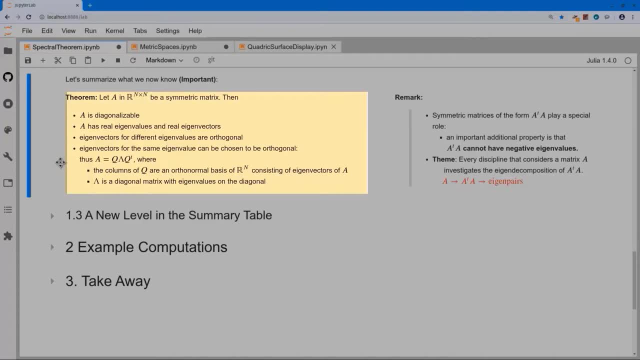 And so we can make them orthogonal And, as a consequence, A is equal to Q lambda times Q transpose where the columns of Q are these orthonormal eigenvectors that now form a basis for Rm, And the lambda matrix is our diagonal matrix of eigenvalues, as before. 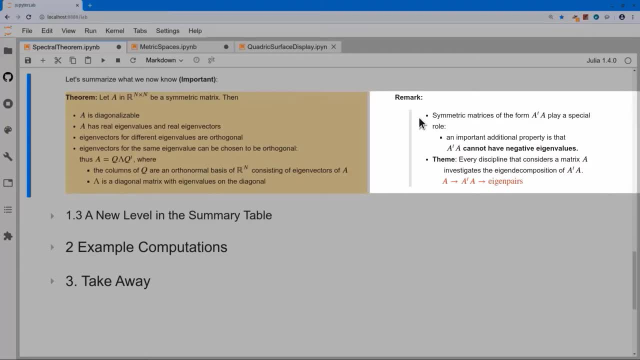 Now a remark to make is that symmetric matrices of the form A transpose A play a very special role In addition to being symmetric. if that symmetric matrix I started with happened to be some matrix, transpose times that matrix, if it looked like that, an additional 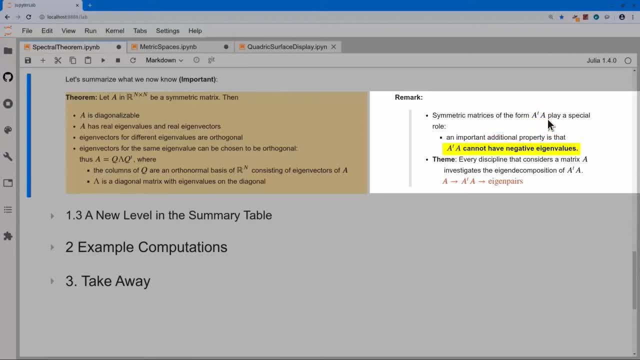 property that that matrix has is that it can't have negative eigenvalues. All the eigenvalues are either zero or positive, And what you'll see in any discipline that deals with matrices is, sooner or later, they find that A transpose A is an interesting matrix, that they end up with symmetric A. 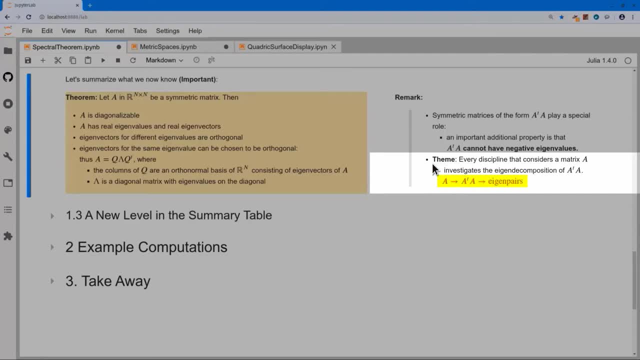 and then immediately compute A, transpose A and then do an eigendecomposition. So it starts with symmetric A, forms A, transpose A, computes the eigenpairs and then assigns meaning to those special directions to the eigenvalue. So then they walk directly into matrix A. 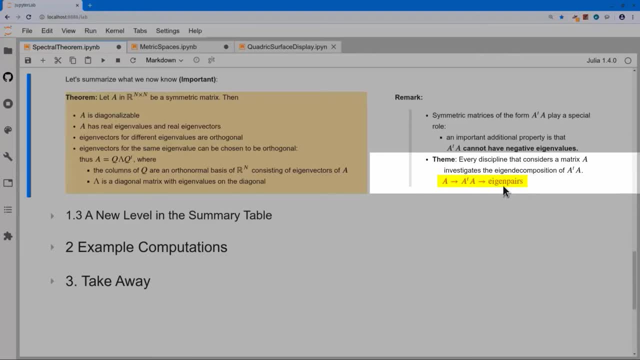 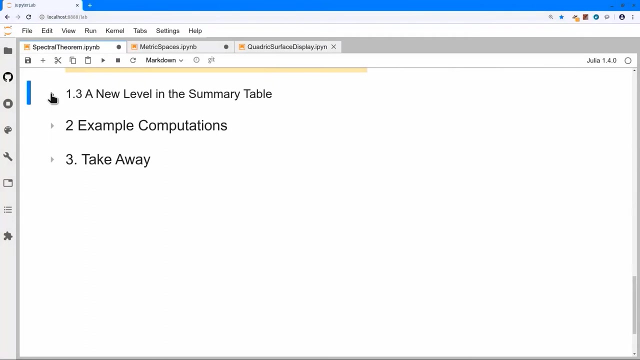 eigenvector directions within the application that actually resulted in that matrix. So you'll see this progression going from A to A transpose A to compute the eigen decomposition of A transpose A. You'll see it everywhere. So now I have a new level in the summary table when I do computations. 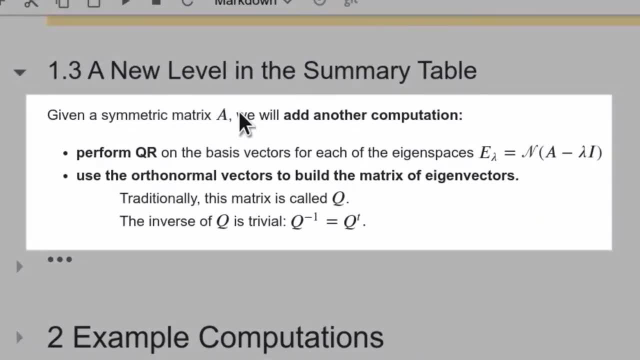 Basically I start with a matrix A and I'll do my eigen decomposition. And once I'm done with that eigen decomposition I'm going to do QR on basis vectors for each of the eigenspaces separate And once I have those new orthonormal basis vectors for each one of those eigenspaces. 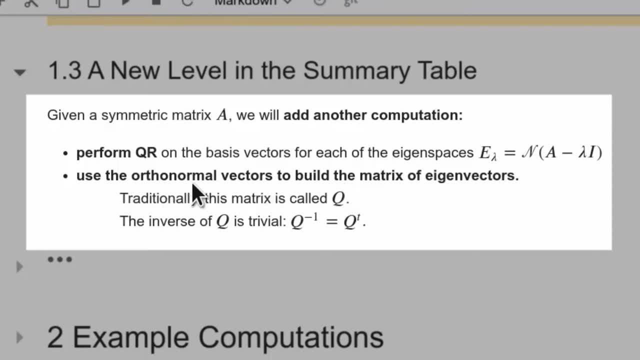 I'm going to use those to build my matrix of eigenvectors. So instead of S from the original vectors, I'm going to form a matrix called Q from the orthonormal eigenvectors, And the important thing to remember is that its inverse now is trivial. I've done extra work. 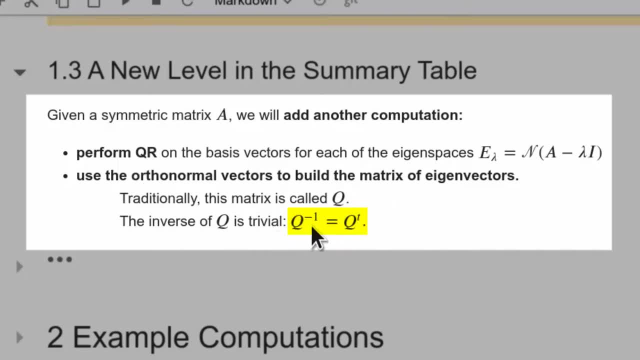 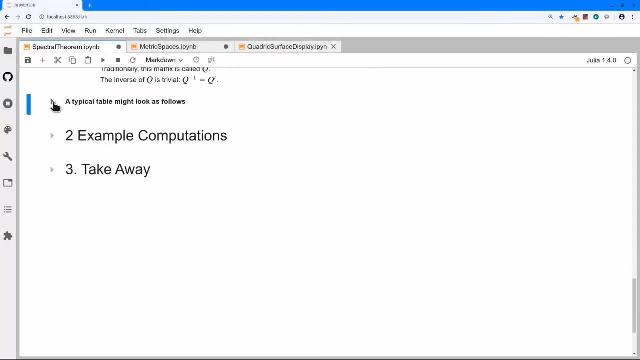 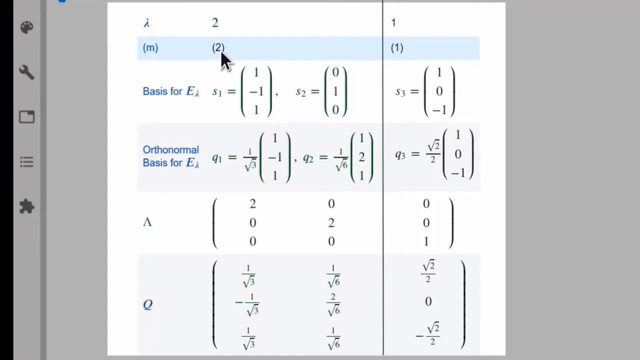 I'm doing QR, but I no longer have to do work to compute the inverse. The inverse is just the transpose of that matrix. So here is what a typical table might look like. I have my eigenvalues as before: Lambda equals two occurred twice, Lambda equals one occurred once, And the corresponding eigenvectors for lambda equals. 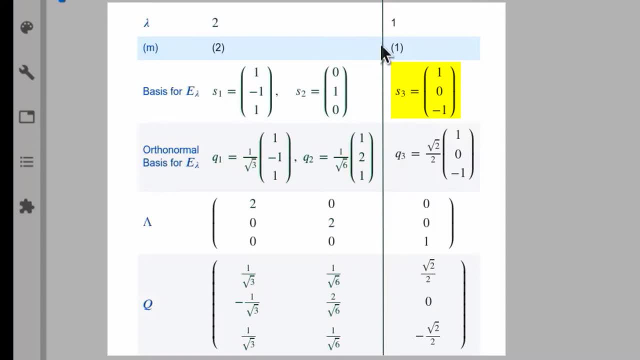 two. I have S one and S two, And for lambda equals one, I have S three. So we have to do gram-sharp, We have to do gram-Schmidt, on eigenvectors S one and S two, corresponding to eigenvalue lambda equals two. 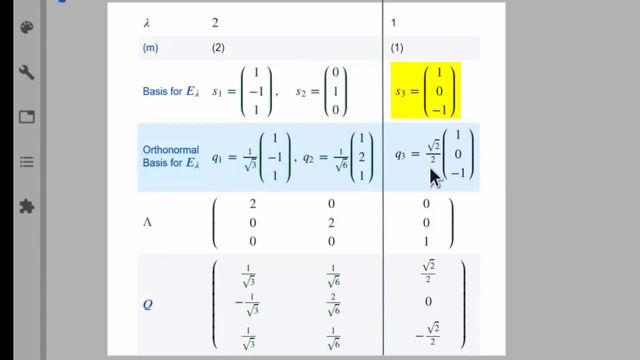 two vectors, And we also have to do gram-Schmidt on eigenvector S three, which corresponds to eigenvalue. lambda equals one, And for a single vector it's just scale the vector to unit length. We then assemble the lambda matrix as before, But when it comes to assembling the eigenvectors, 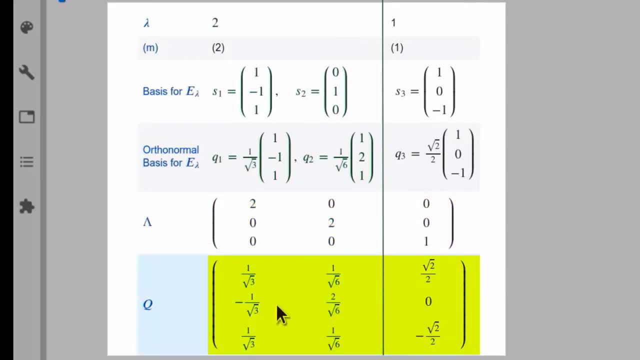 we are going to assemble them from the orthonormal vectors, from the Q vectors. So we are going to copy down the Q one and Q two vectors for eigenvalue two and the Q three vector for eigenvalue three. Now, if you look at our computations here, 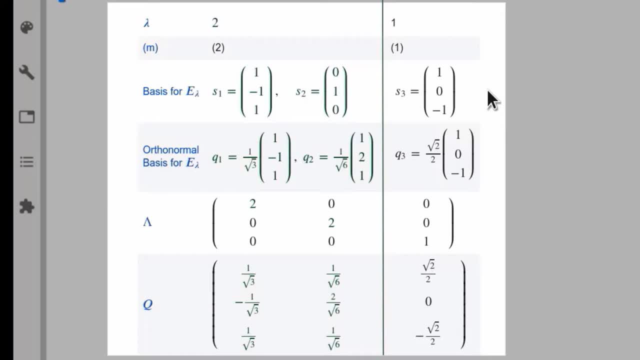 the idea was that this starts from a normal matrix, so from a symmetric matrix in this case. So the eigenvector for lambda equals one must be orthogonal to the eigenvectors for lambda equals two. And if you check the dot products, the dot products of S three with S two is equal two. 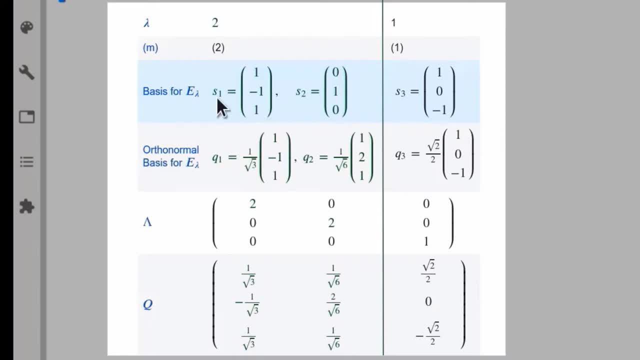 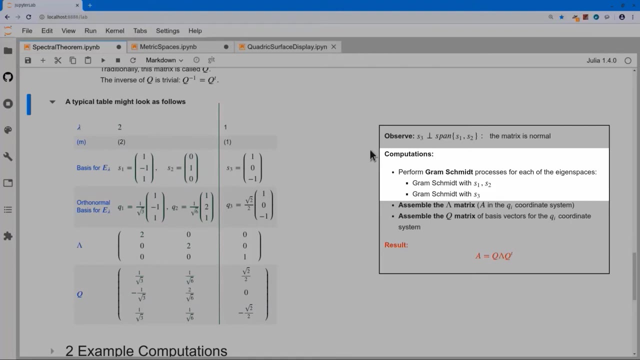 to zero and the dot product of S3 with S1 is equal to zero And, as a consequence, the dot product of S3 with any linear combination of these two vectors. any other eigenvector for lambda equals two is also equal to zero. And to repeat the extra computations, we are now 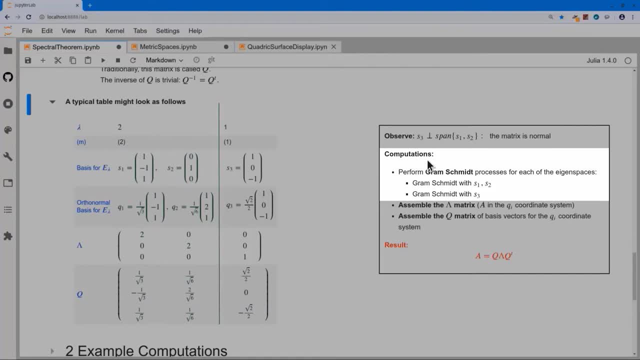 performing is: we do our eigen decomposition as before, but then we do Gram-Schmidt for the eigenvectors associated with each of the eigenvalues separately, And once we have done that, we are assembling the lambda matrix as before, And the lambda matrix is just the matrix. 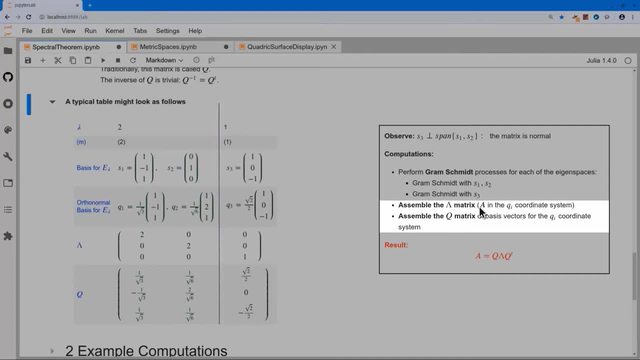 A in our Orson-Normal set of basis vectors, or it would also be the same matrix A in our other set of basis vectors, It doesn't really matter which set of basis vectors we take. And we assembled not the S matrix but the Q matrix from the Orson-Normal vector And the result is that we get 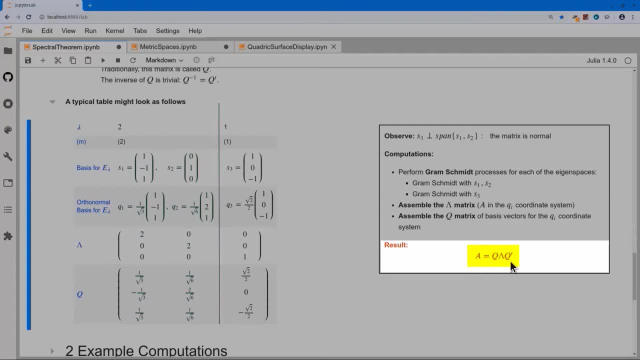 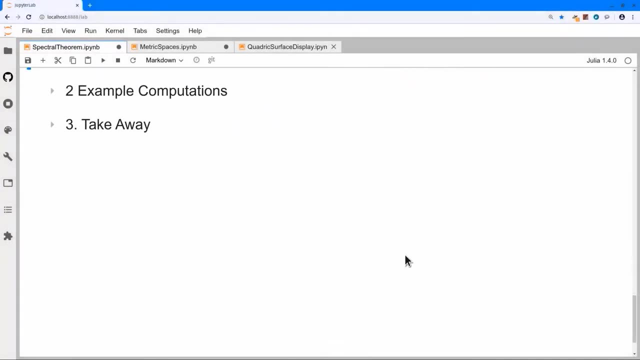 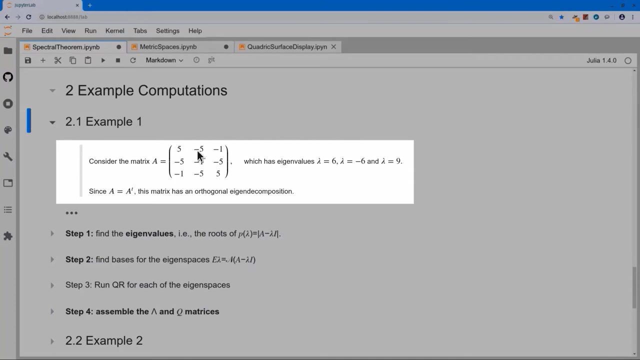 A equal to Q times lambda, times Q inverse, And the result is now simple: It's Q transpose. So let's see how example computations might run. My first example is: I have this matrix and if you look at it you see that, yes, it is symmetric. 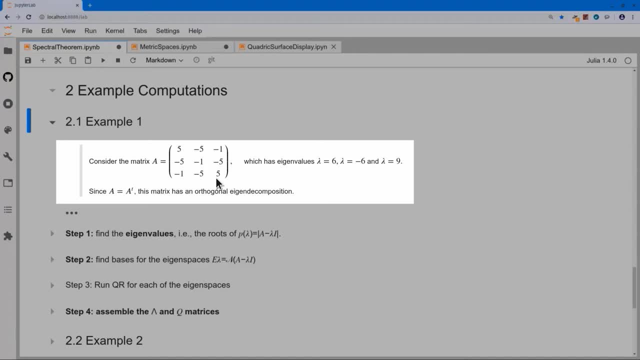 and therefore we know we're in business. We can find an orthogonal eigen decomposition for this matrix And it has eigenvalues. lambda equals six minus six and nine, which, well, I wouldn't get them by hand very easily, but I certainly get them with a computer. 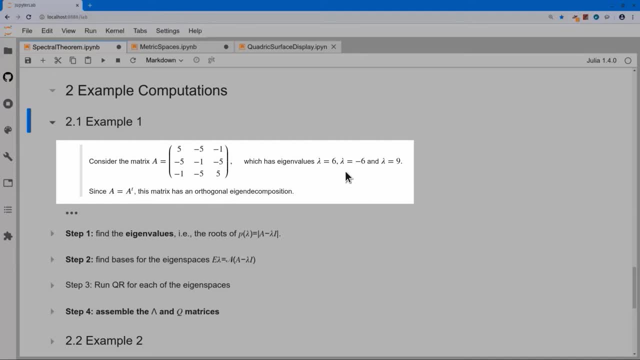 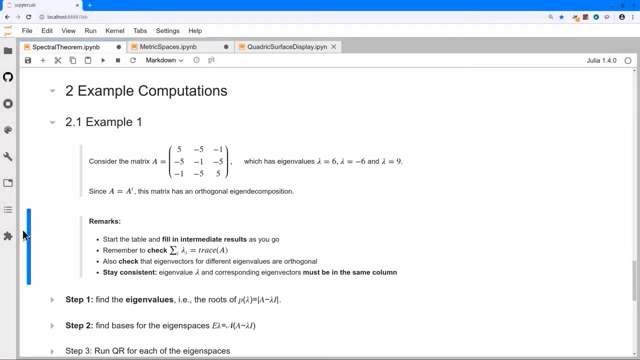 And I know that I am in business, that not only do I have an eigen decomposition, but that the unit vectors corresponding to these three eigenvalues are going to be automatically orthogonal, and all I will have to do is scale their lengths. So let's see how this goes. One thing I'll do if I do these computations by hand is 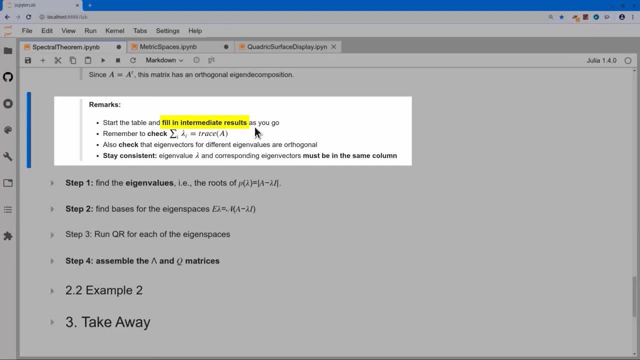 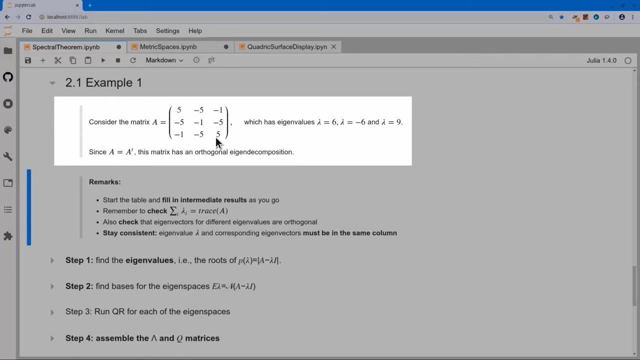 I'll start that table and I'll fill in all of the results as soon as I have them. And remember, I want to check my trace formula. I want to check that the eigenvalues indeed add up to the trace of the matrix. So let's quickly see: five minus one plus five is nine. 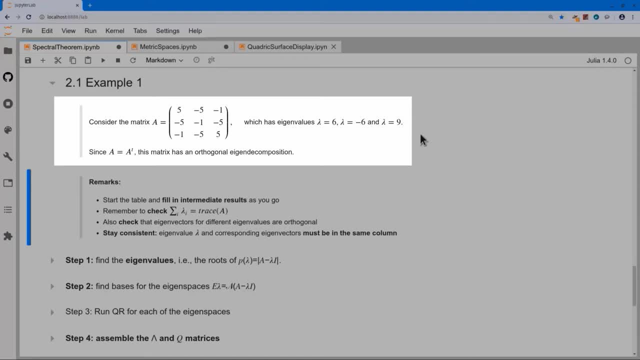 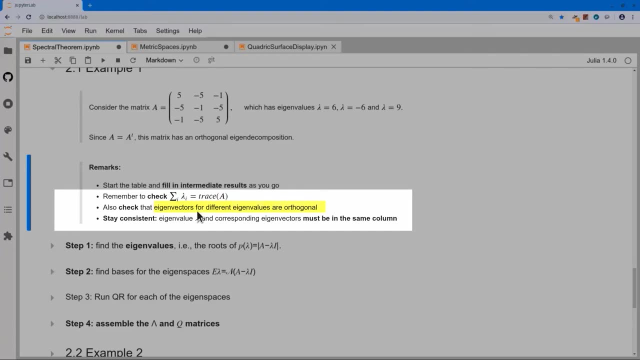 six minus six plus nine is nine. So okay, it looks like I have the right eigenvalues here. my trace formula is satisfied, And the other thing I might want to do is to check that the eigenvectors for different eigenvalues are indeed orthogonal by doing the dot products. The other point to make is: 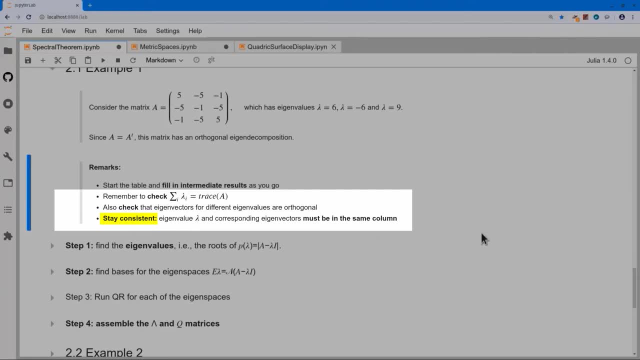 to check that the eigenvalues are consistent with our table. Whenever we fill in an eigenvalue, the corresponding eigenvectors must be right then and easily in the same column, And I'll emphasize it again when we look at the table next. So our first step: we need to find the eigenvalues. 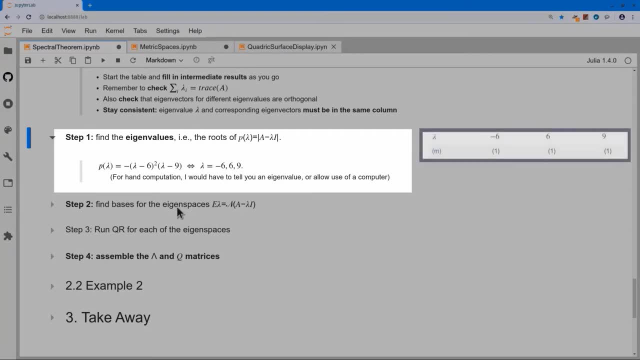 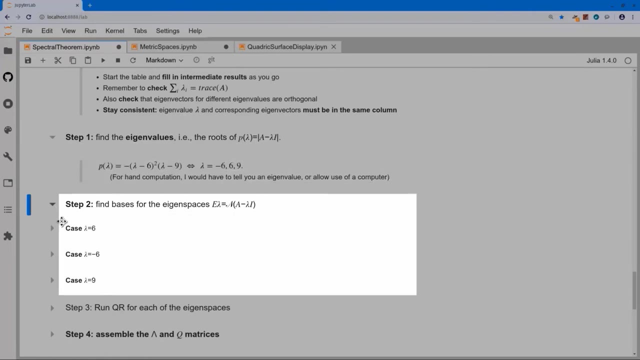 and we found them somehow. lambda equals minus six, six and nine, And therefore step one is complete. we have the eigenvalues. Now we have to find the eigenspaces, So the null spaces of A and the I, And there are three cases to consider: lambda equals six, lambda equals minus six and 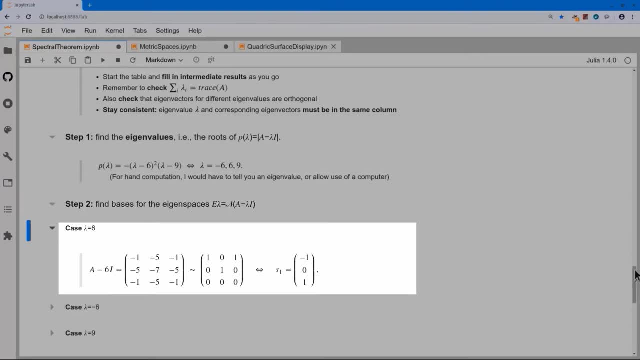 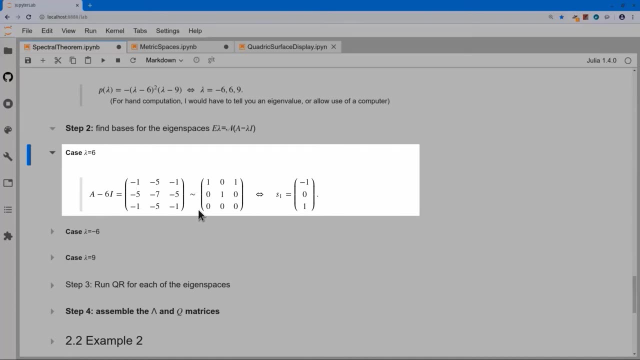 lambda equals nine. So for lambda equals six, we look at A minus six I. we find this matrix here, we do Gaussian elimination. it results in a single missing pivot, as we knew we would have, since the dimension of the eigen space is known to be one, And solving for the homogeneous solution. 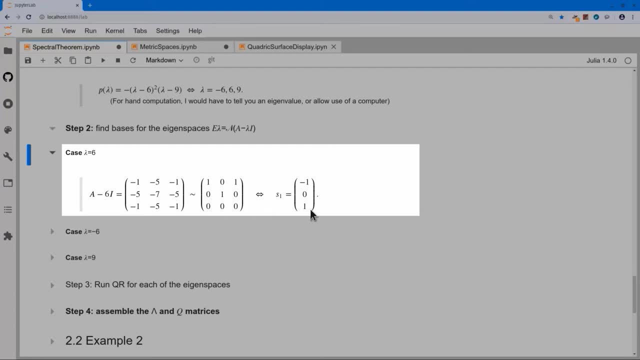 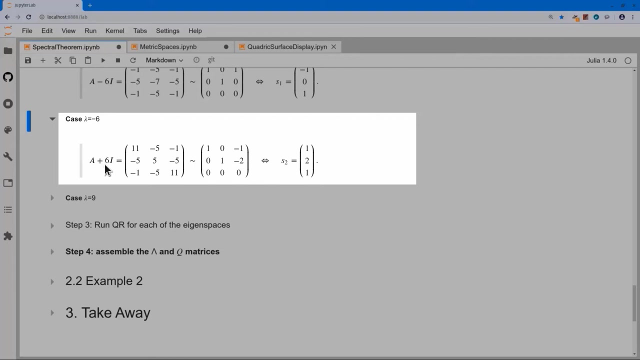 here we find a single vector minus one, zero one, As a basis vector for the null space of A minus six. I Now for lambda equals minus six. the computation is similar. So we have to look at A minus lambda I and lambda is negative, so A plus. 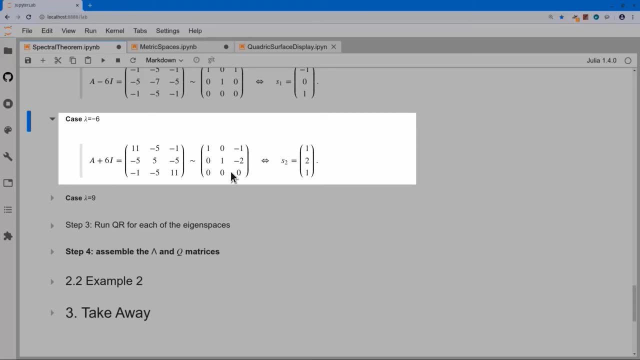 six I, Gaussian elimination yields a missing pivot again And we have an eigenvector basis for the null space of A plus six I consisting of this vector here And we immediately check the dot product between this one and the other And we immediately check the dot product between this one. 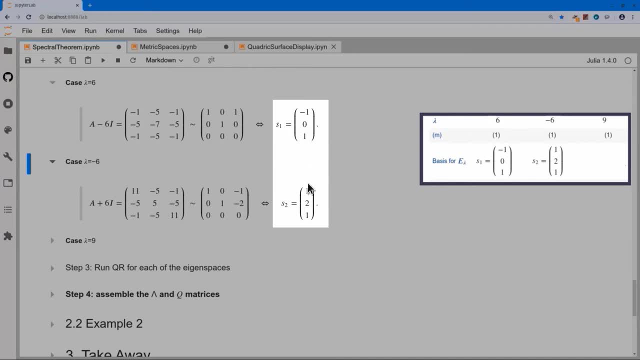 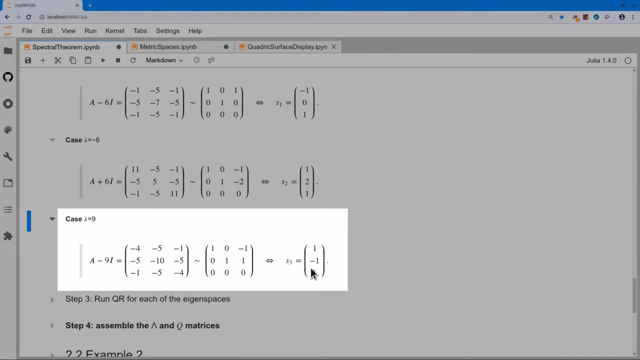 and this two is indeed zero. Those two vectors are orthogonal, as our spectrum theorem said they would have to be. Finally, case lambda equals nine is similar. We take our matrix, we do Gaussian elimination to find our missing pivot, We find a new eigenvector And if you do the dot products, 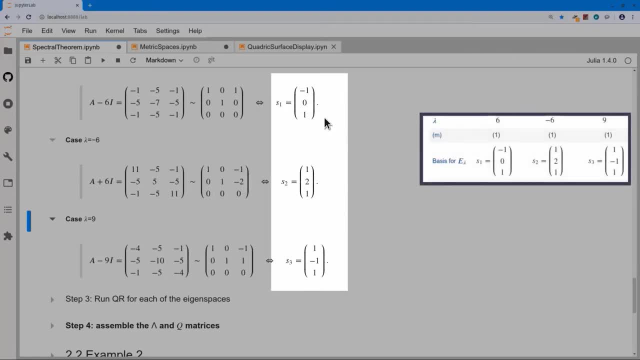 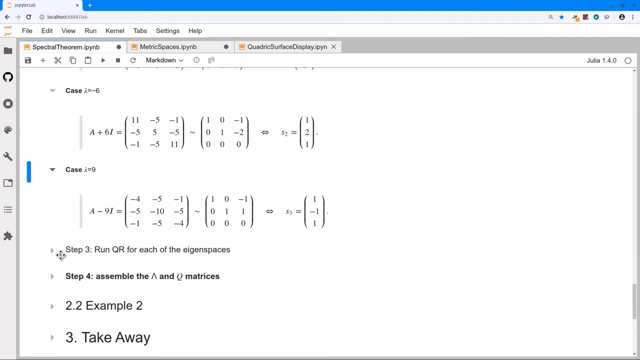 between S three and S two and S three and S one, we find that they're zero. So these eigenvectors, these three eigenvectors, are orthogonal from the outset. My next step is to run QR. Well, QR, in each eigen space, simply says scale that vector to unit. 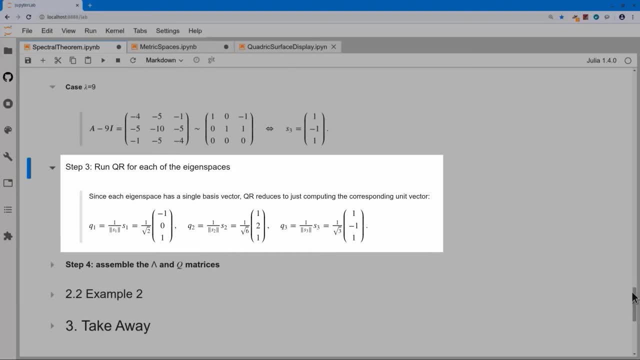 length. That's the only formula that's left, That's: W one is equal to S one, Q one is one over the length of S one times S one. Scaling them, we have scale factors of square root of two, square root of six and square root of three coming in. And now, when we assemble all of our matrices, here's what. 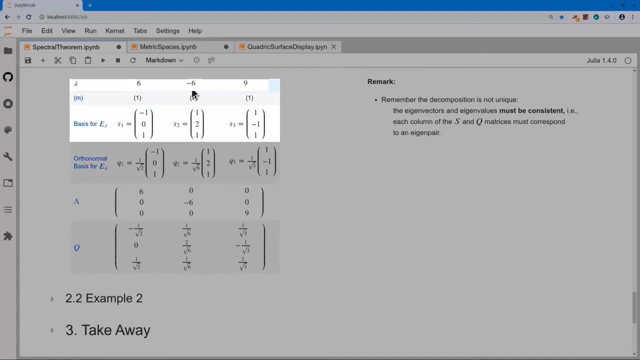 the table looks like We have three different eigenvalues. We have two different eigenvalues. One is six, six, nine. The multiplicities for each one of them were one. So we knew we had a single eigenvector in the basis that we were going to find. So for eigenvalue plus six, remember to 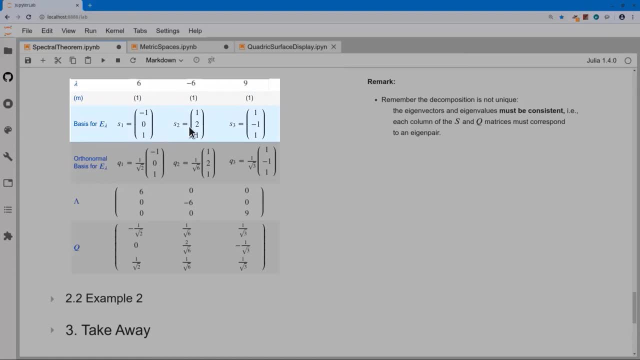 write it right underneath: Eigenvector S one For minus six. eigenvector S two For plus nine. eigenvector S three. Then we do Gram-Schmidt for each one of the eigenvalues. So for lambda equals six. we have a single vector, So we just scale to unit length. 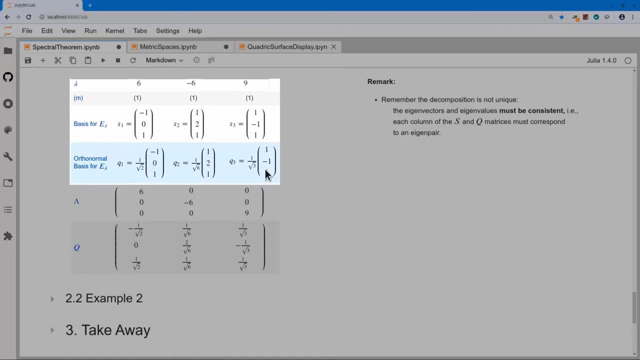 Similarly for lambda equals minus six, lambda equals nine, And when we assemble the matrices, the eigenvalues just copy down in the same order as above, So six minus six and nine And the eigenvectors: we're pulling our orthonormal eigenvectors and copy those down. And so here is. 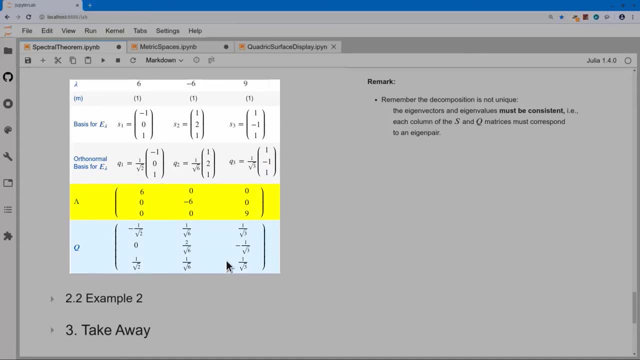 my lambda matrix and my Q matrix. for A equals Q, lambda, Q transpose. Now remember that the eigendecomposition is not unique. How we order the lambdas and how we order vectors within an eigenspace is arbitrary. So if you and I did the same problem and wrote different orders of the lambdas down, 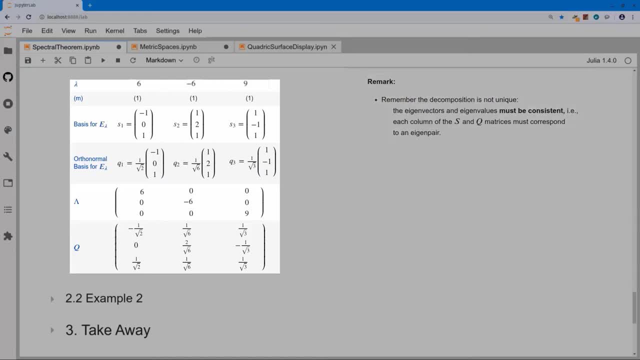 we would get a valid eigen decomposition. And when we multiply out our eigen decomposition- q times lambda, times q transpose, we both get A as before. All that is required is that we be consistent, That the matrices that we copy down and the vectors that we copy down and the 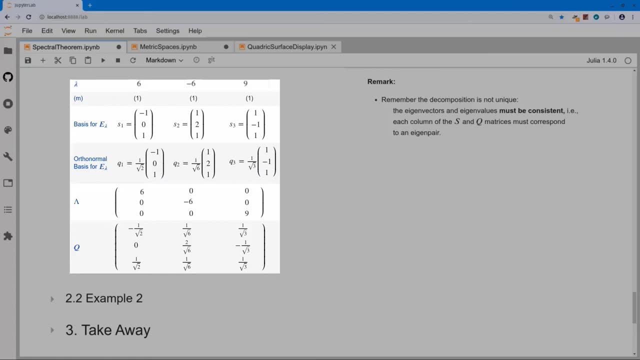 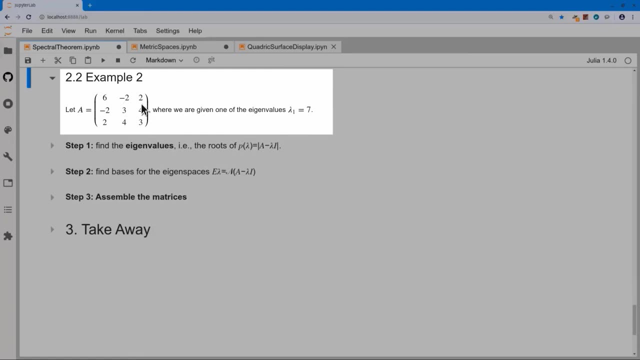 eigenvalues that we copy down must belong together. For our second example, we'll look at this matrix here: 6 minus 2 and 2.. And this time around I'll actually make it a little bit more involved. I'll say: I'll give you one of the eigenvalues, somehow or other. I know an eigenvalue, I know it's equal. 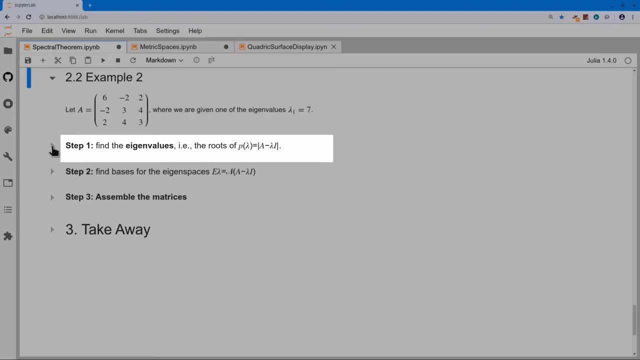 to seven. So my first step is to find the eigenvalues, and of course I could also find the eigenvalues. I could also find the eigenvalues in the matrix, compute the polynomial and divide out lambda minus 7.. But since I had that, I can do a little. 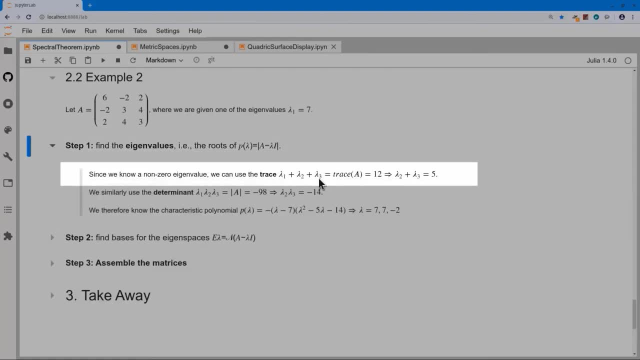 bit better. We know what the trace is. Lambda 1 plus lambda 2 plus lambda 3 is equal to the trace of A. The trace of A 6 plus 3 plus 3 is equal to 12.. And therefore from lambda 1 equals 7. 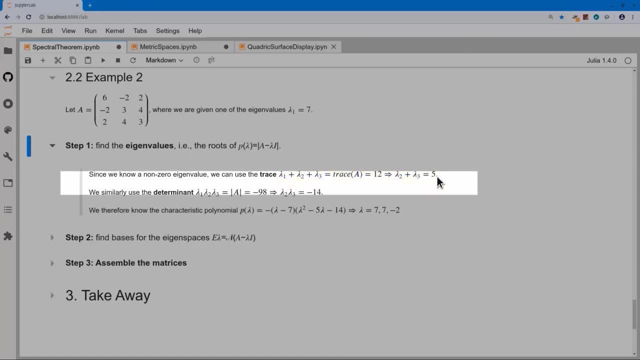 plugging in, I know lambda 2 plus lambda 3. They add up to 5. If I compute the determinant of A, I find minus 98. I'd probably use Gaussian elimination, at least one step of it, to make. 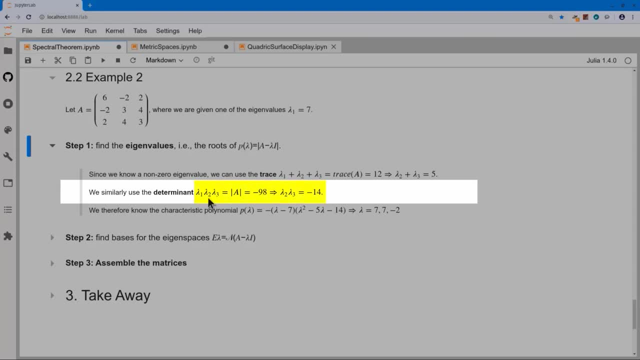 it easier Once I have the determinant, since the determinant is the product of the eigenvalues. dividing out lambda 1, that we know is 7, we get that lambda 2, lambda 3 is equal to minus 14.. So we know the characteristic polynomial. We have a minus sign because our matrix is 3 by 3,. 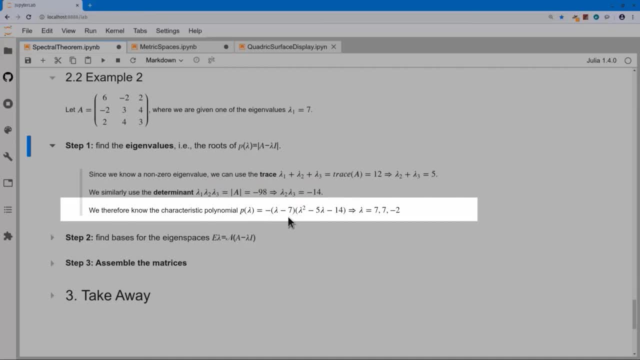 so minus 1. to the third power They factor lambda minus 7, since 7 is an eigenvalue. And then the remaining polynomial is a factor: lambda squared minus the trace of the remaining eigenvalues minus 5. lambda plus the product of the remaining eigenvalues plus minus 14.. And solving for the roots of that, 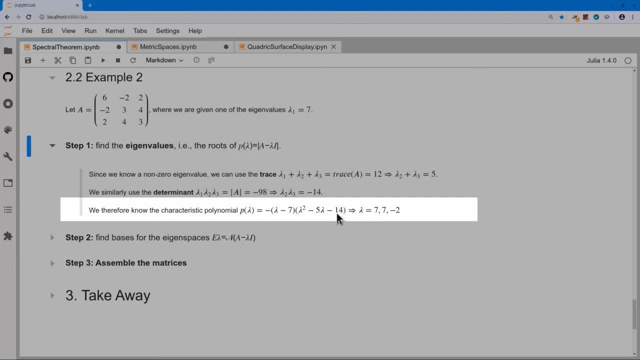 quadratic polynomial, I find 7 and minus 2.. So now I've got my three eigenvalues: 7 repeated twice and minus 2.. The next step is to compute the non-space spaces, Non-space of A minus lambda I and I have two cases. 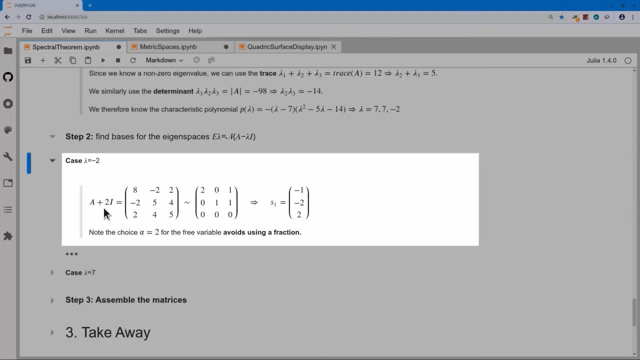 If I compute A minus lambda I, for lambda equals minus 2, I get after Gaussian elimination. I have a missing pivot, as I knew I would, because the multiplicity was 1. And the basis for that null space that I picked out is minus 1, minus 2, 2.. Notice that compared to the normal way of doing. 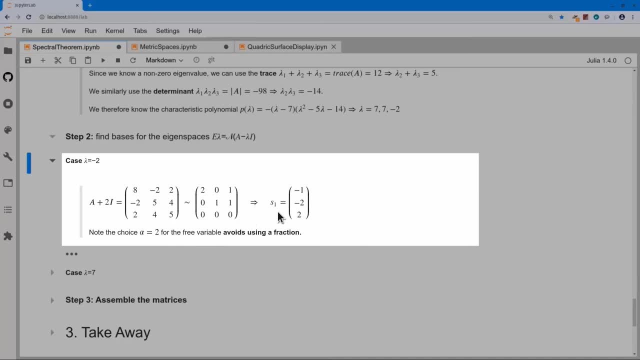 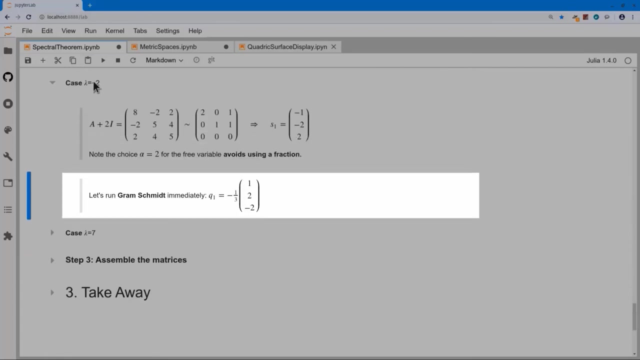 things. I chose to use alpha equal to 2, because that made the fraction go away. We're going to scale this vector to unit length to begin, But whatever length we use, it really doesn't matter. to get in decomposition, Let's do Gram-Schmidt right away. We have to do Gram-Schmidt for this eigenvalue. 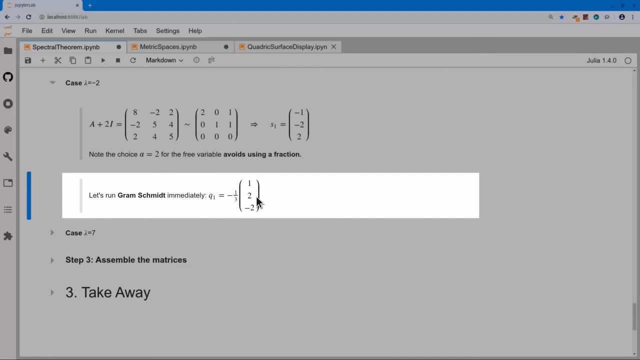 single vector, And so it's just scale that vector to unit length. Norm squared is 1 plus 4 plus 4, 9, so 1 over minus 3.. I pulled out the minus sign simply because I like one less minus sign. 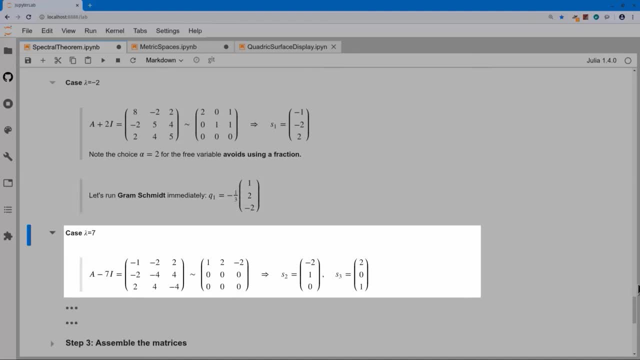 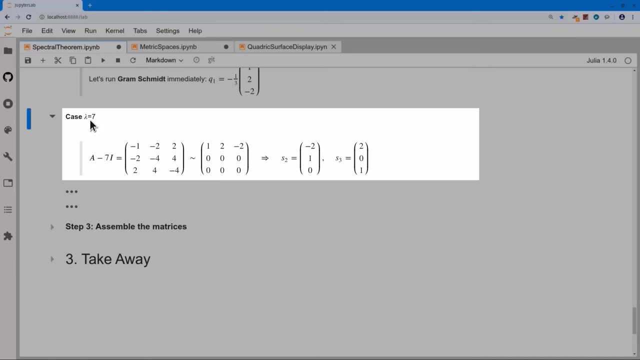 going to be minus 3.. So we know that it's going to be minus 3.. So we know that it's going to 7 occurred twice. so we know we have to find 2 eigenvectors. Here's my matrix: Gauss elimination, indeed, finds 2 missing pivots, And writing down. 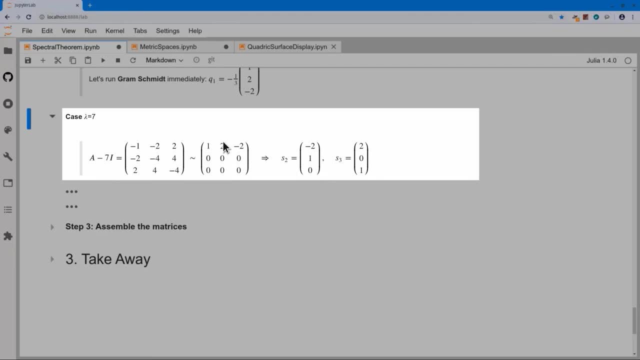 the eigenbasis is trivial, since we have a single row, It's 1,. 2 interchange 1 sign, change so minimum 2.. 1 and 1 minus 2 interchange those two values and change 1 of the signs to 1, and everything else is 0.. 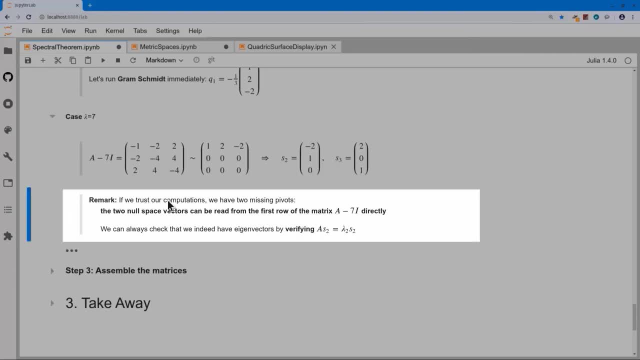 The point, however, is that if I trust my computation, if I think yes, lambda equals seven is correct, then I know I'm going to have two missing pivots, I know I'm going to have zeros underneath, I know I'm going to end up with just this single row from the outset. 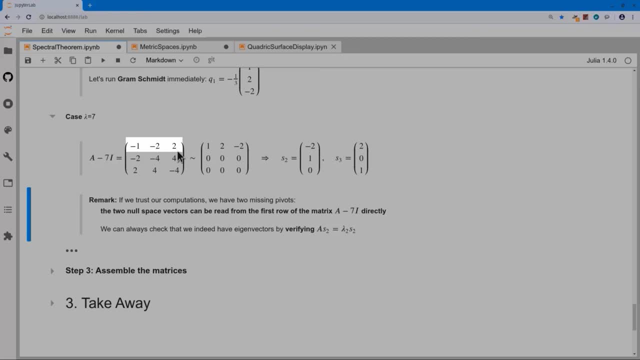 And so just this single row is what defines my eigen space. So I don't have to do Gaussian elimination, I don't have to do that extra computation. I can just read off the null space from that first row and get the exact same answer that I've written down before. 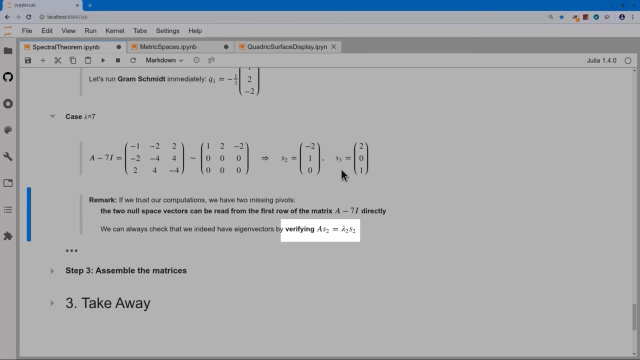 I said, if I trust my computation, I could still do it, and then simply check whether or not these are indeed eigenvectors, whether or not a times that vector as two gives me seven times that vector as two. So I can always check. 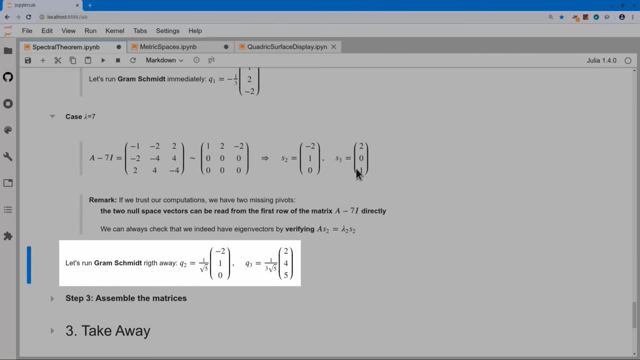 Now the last step is: again, I'll do Gram Schmidt. This time I have two vectors to do Gram Schmidt on, So the first vector gets scaled to unit length And the second vector. I'll have the Gram Schmidt equation for two vectors and scale to unit length, And so I get q2 and q3. what? 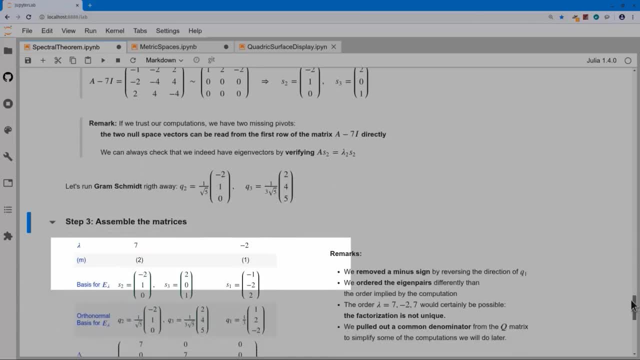 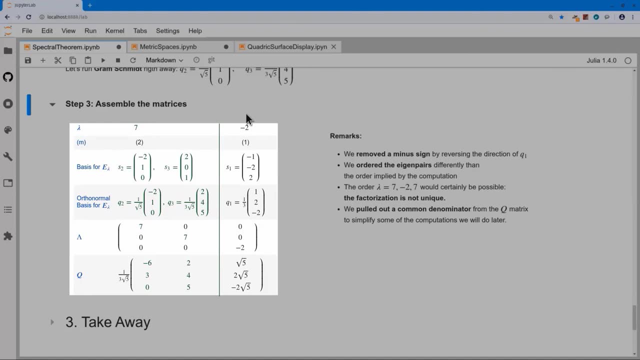 We have plugged in the values as we went, But here is the end result. when I put my table together, I have an eigenvalue seven which occurs twice, and an eigenvalue minus two which occurred once. Then, for eigenvalue seven, we found 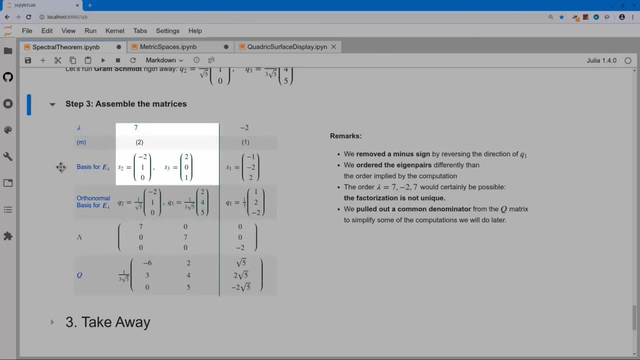 two eigenvectors. So I wrote in the s vectors s two and s three, and for eigenvalue equal to minus 2, my lambda 1 eigenvalue, what I called it before, what the index had chosen before I found the vector S1.. And what I have to do now is I have to do a grand schmidt for each of the. 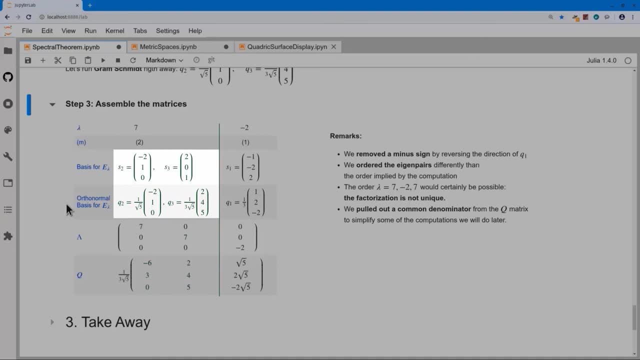 eigenvalues. So S2 and S3 belong together. QR on those. S1 belongs to eigenvalue minus 2, so QR on just S1.. And finally, assembling my matrices, assembling the lambda matrix by copying down the eigenvalues. 7 occurred twice and so I have it twice on the diagonal. And finally, the Q. 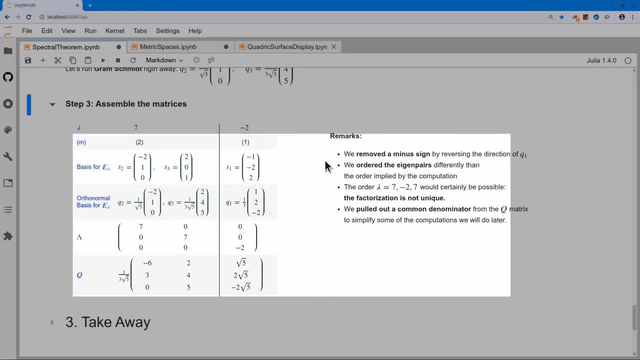 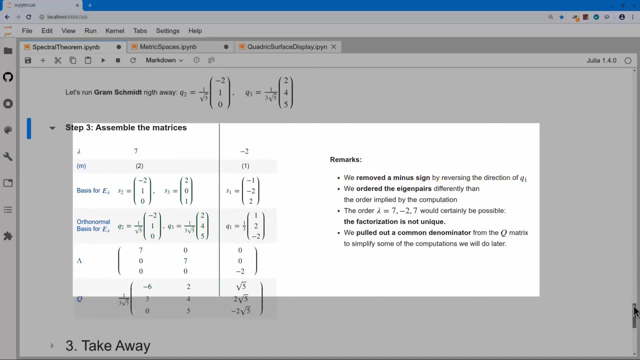 matrices. I have to copy down the Q values. Now some comments on what I did. here. is I removed a minus sign by reversing the direction of Q1.. If you remember Q1, Q1 is minus 1, third times 1,. 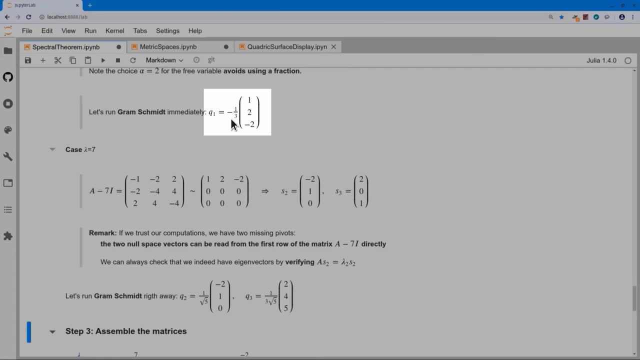 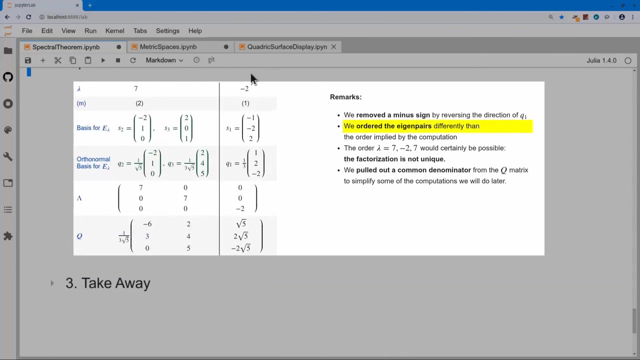 2, minus 2.. Well, I just need an orthogonal direction. I and minus I are orthogonal to J itself. I can change the direction of the vector. I can drop that minus sign if I choose, And here I chose to do that. The other thing is I ordered my eigenvectors and eigenvalues differently than 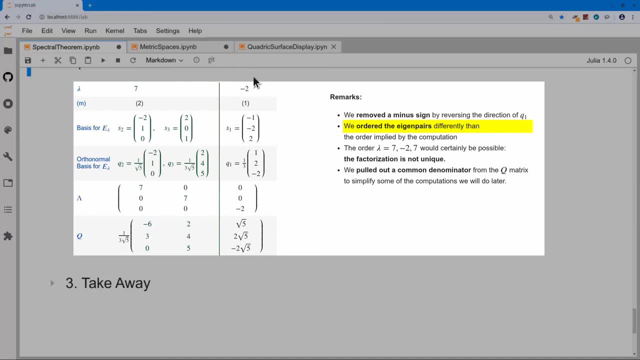 the order in which I did my computation, just to show that I could. So I chose to write lambda equals 7 first, and then lambda equals minus 2 second, and assembled my matrices accordingly. Remember, I just had to make sure that I stay consistent, that I copy things down in the same 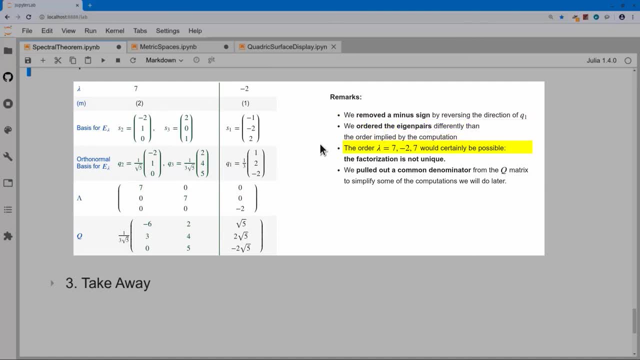 order. Could I do other orders, Of course. For example, I could split lambda as 7, minus 2, and 7.. I don't know why I would do that, but I could if I chose to. The factorization is not unique. 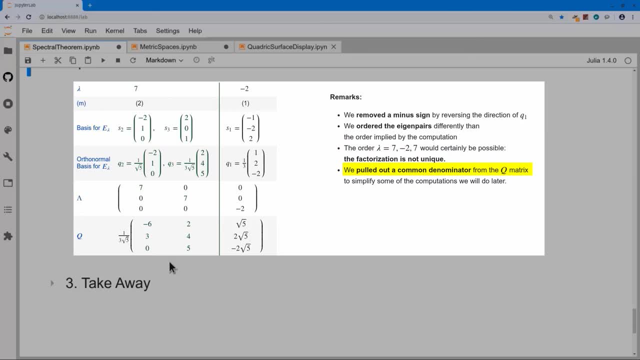 The last point I want to make is look at my matrix Q. I chose to pull out the common denominator. I chose to pull out 1 over 3 times square root of 5, so that I don't have any nasty denominators in. 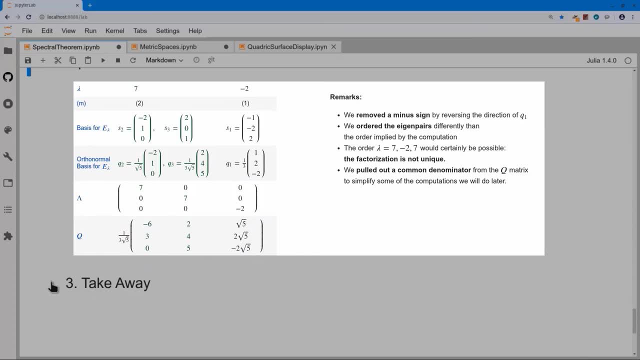 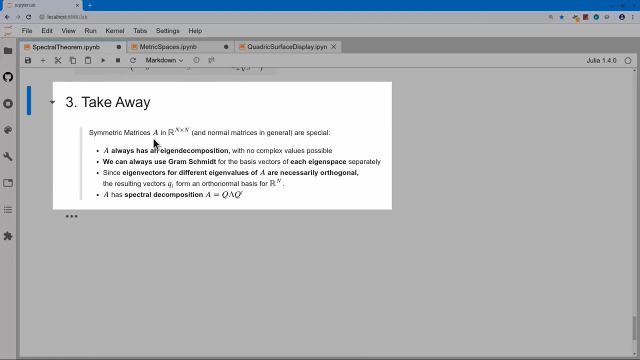 my matrix itself. So our takeaway for today for the spectral matrix: what happened to it? What we have done is we found that symmetric matrices are quite special and normal matrices in general are quite special. They always have an eigen decomposition. There are no complex values. 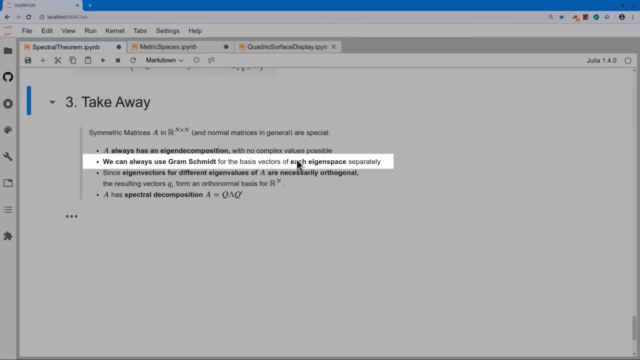 We can always use Gram-Schmidt to make the basis vectors in each eigenspace orthonormal. The eigenvectors for different eigenvalues of A are necessarily orthogonal, so there's nothing special I need to do for those. I'm going to end up if I do this process. 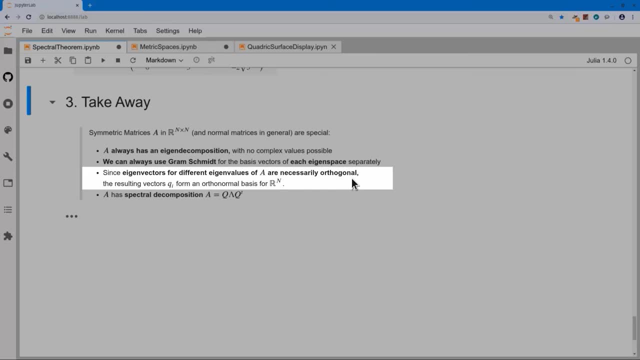 if I run Gram-Schmidt on each of the eigenspaces, I end up with an orthonormal set of eigenvectors. Therefore when I write down the spectral decomposition with that set of basis vectors, with the orthonormal basis vectors, the inverse of Q is just Q. transpose My decomposition.